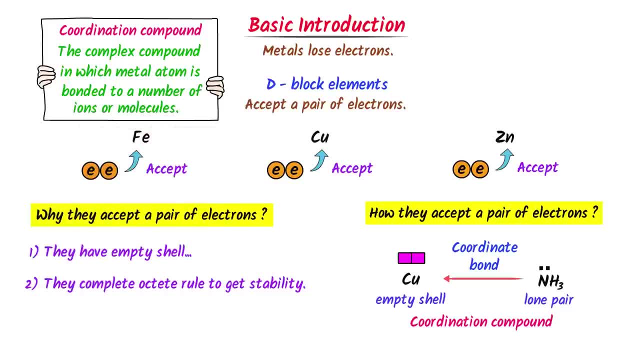 Let me repeat it: The complex compound in which metal atom is bonded to a number of ions or a molecule is called coordination compound. Remember that this NH3 donate a pair of electrons to a metal atom. We call it ligand. So we define ligand as: 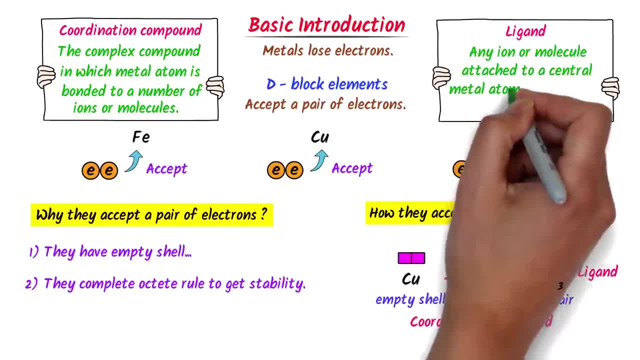 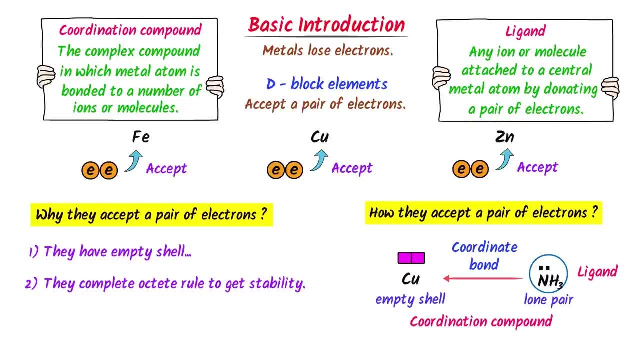 any ion or molecule attached to a central metal atom by donating a pair of electron is called ligand. Thus, remember that any coordination compound is made up of two parts. One part is a metal atom like copper, and the second part is a ligand. 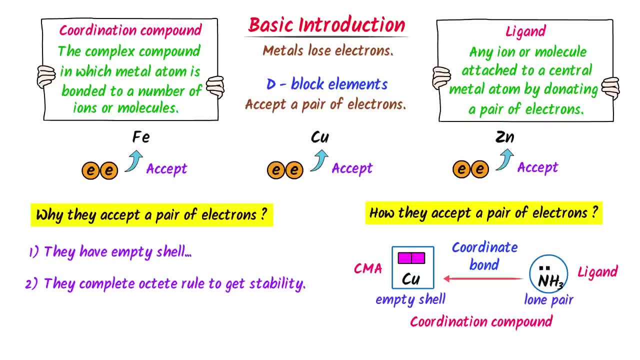 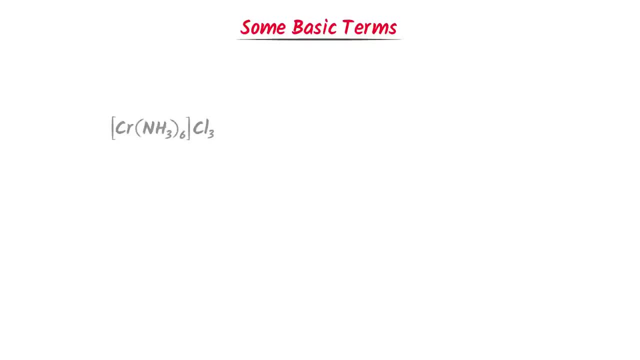 Like NH3.. Thus noted down all these important points, Now let me teach you some basic terms of coordination compounds. Let consider this coordination compound. There are three species in this coordination compound: Chromium, NH3 and chlorine. Now listen carefully. This metal atom of chromium is known as central atom. We know that NH3. 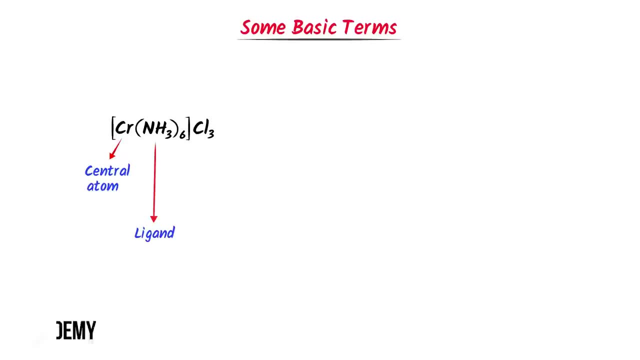 donate a pair of electrons. Chromium is a ligand. This six means six molecules of NH3.. One molecule of NH3 donate one pair of electrons. Six molecules of NH3 donate six pair of electrons. We call this six as coordination number. Remember that coordination number shows the number of pair. 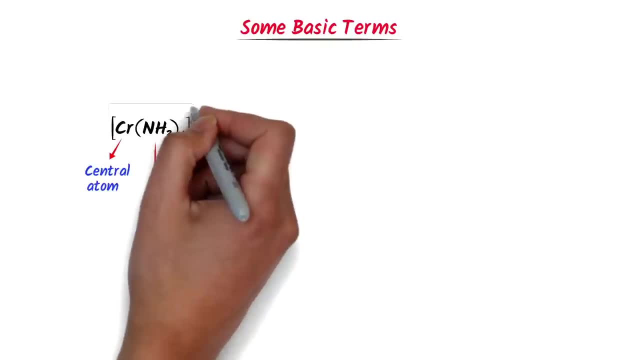 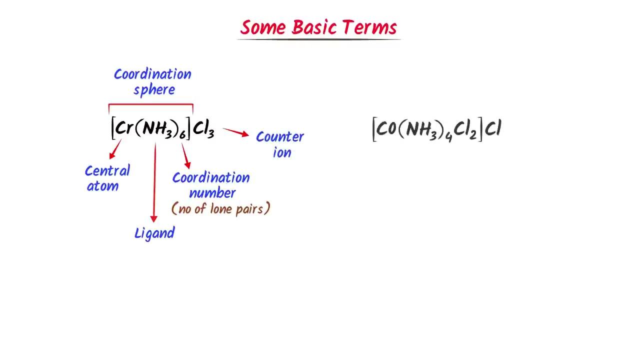 of electrons donated. This chromium, NH3 and the square bracket is called coordination Sphere or coordination entity. This chlorine outside the bracket is called counter ion. Secondly, consider this complex compound. Here cobalt is a metal atom and we call it central atom. This chlorine is ligand. This two is the coordination number of chlorine. This 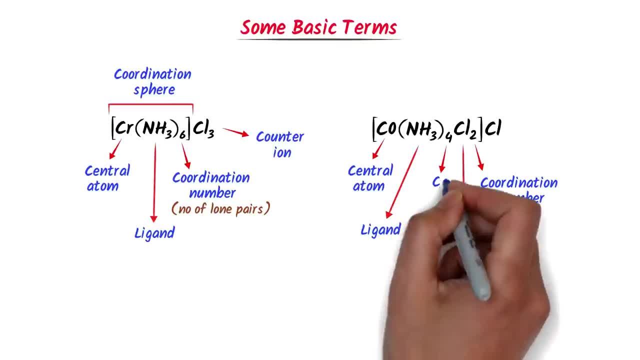 NH3 is another ligand and this four is its coordination number. This whole thing and the square bracket is known as coordination sphere or coordination entity. This chlorine outside the square bracket or coordination sphere is called counter ion. Thus noted down all these basic terms of coordination compounds. 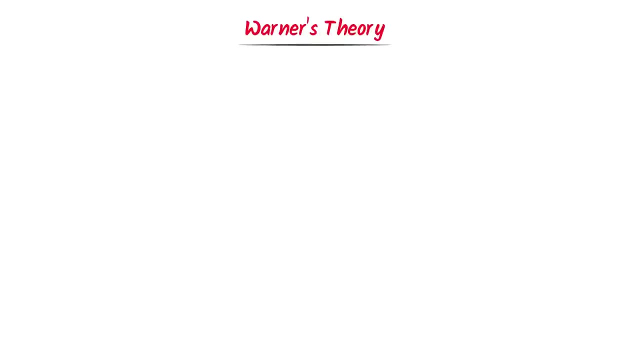 Now let me teach you Warner's theory. Well, Warner is the first scientist who successfully studied coordination compounds. He took cobalt chloride and he reacted a different way. He started with NH3.. After reaction, he got cobalt chloride dot 6, NH3.. Secondly, he added: 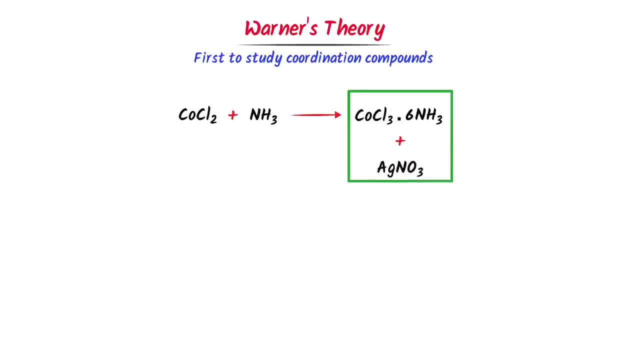 silver nitrate to cobalt, dot 6 NH3.. After reaction he got three moles of AgCl3 or silver chloride in the form of white precipitate or white PPT. Now listen carefully: Warner and Warner are directly bonded to cobalt and 6 NH3 strongly are directly bonded to cobalt. 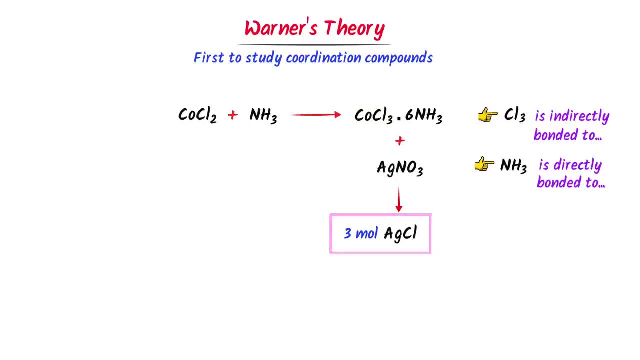 That's why chlorine love to react with silver. So he rearranged this compound. He writes the central metal atom of cobalt, Then he takes NH3 and there are six molecules of NH3. He puts square bracket around these two species. Finally, he writes chlorine and there are: 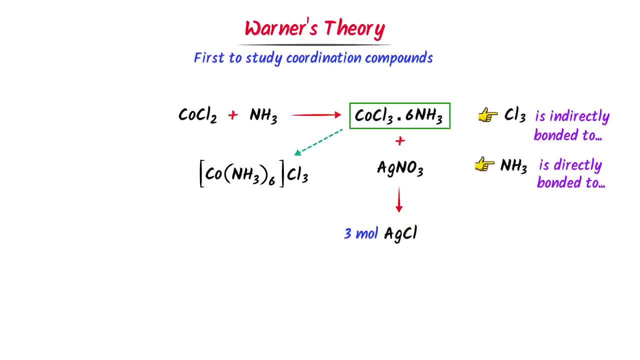 three of them. So Warner-Baba therefore say that 6 NH3 are directly bonded to cobalt and 3 chlorine are indirectly bonded to cobalt. He called this compound as coordination compound. Remember that this is the first coordination compound in chemistry. Now what is the conclusion? 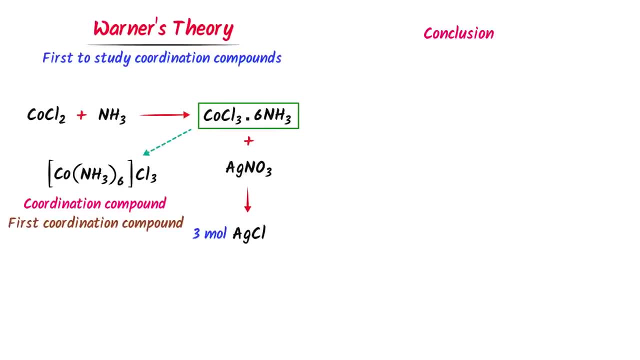 of Warner's theory. Well, Warner-Baba states that every metal atom of coordination compounds has two types of valences. Now, what is the conclusion of Warner's theory? Well, Warner-Baba states that every metal atom has two types of valences: Primary valency and secondary valency. Primary valency is: 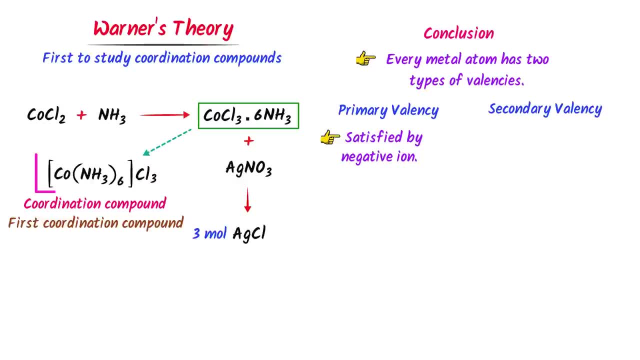 satisfied by negative ion. For example, here in this coordination compound, chlorine is a negative ion. It satisfies the primary valency of cobalt, While secondary valency is satisfied by positive ion or neutral molecule. For example, here in this compound, the NH3 is a neutral. 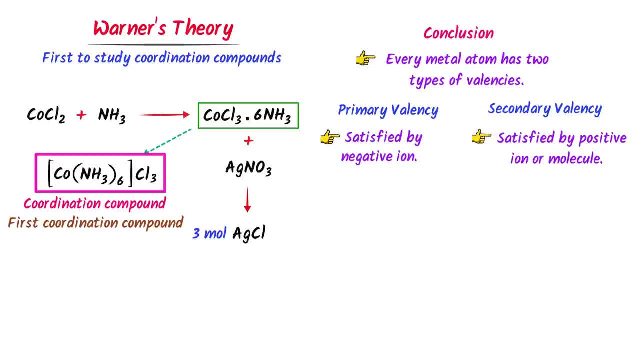 molecule, It satisfies the secondary valency of cobalt. Secondly, primary valency represents the oxidation state of a central metal atom, while secondary valency represents the coordination number. Thirdly, primary valency is denoted by dots and secondary valency is denoted by line. 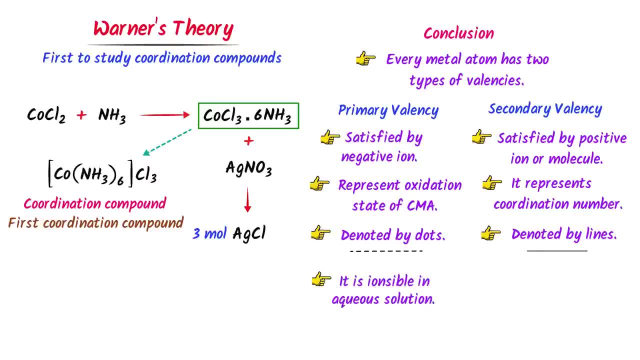 Fourthly, primary valency is ionizable. For example, chlorine is ionizable and aqueous solution, While secondary valency is not ionizable. N3 is directly bonded to cobalt. it is not ionized. Thus noted down all these important points. 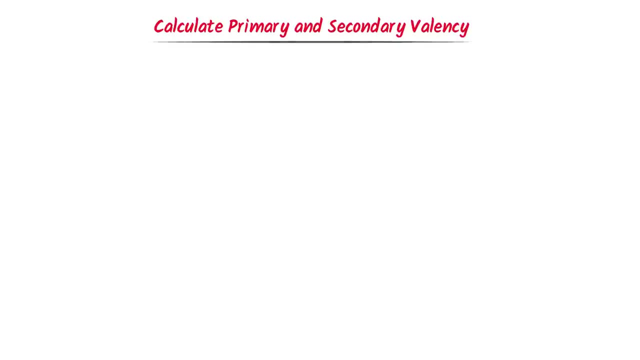 Now, how can we calculate primary and secondary valencies of a central metal atom? Well, consider these coordination compounds. We have already learnt that primary valency is the oxidation number of the central metal atom. secondary valency is the oxidation number of a central metal atom. Primary valency is an oxidation rate that habitually activates. 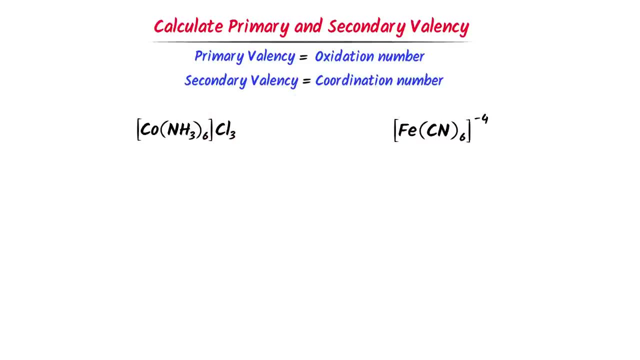 later in the täntri. well, consider these one oneispace singlets. I already said concurrence. the oxidation number of the central metal atom and secondary valence is stopuarum 3 valency is coordination number. Now, in case of this molecule, the central atom is cobalt. 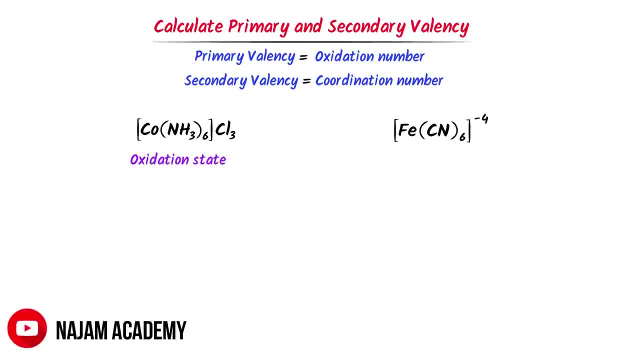 I am going to find its oxidation state. I write cobalt plus 6 and 2. NH3 plus 3- chlorine equals 0. We know that NH3 is a neutral molecule, so its oxidation state is 0 and that of chlorine is positive 1.. So I write: cobalt plus 6 and 2. 0 plus 3 and 2 negative 1 equals 0. After: 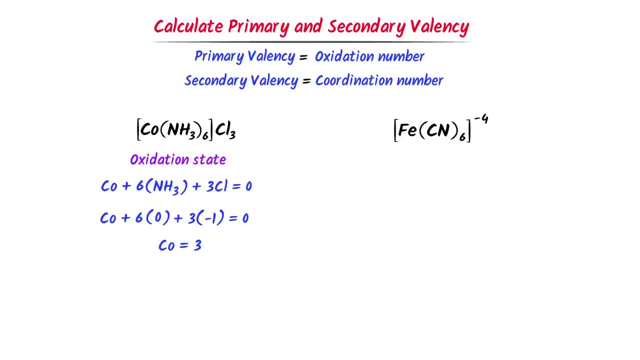 calculation: I get positive: 3.. The oxidation state of cobalt is positive: 3.. So the primary valency of cobalt is 3.. Here we can see that there are 6 ligands of NH3.. So the secondary valency of cobalt is 6.. 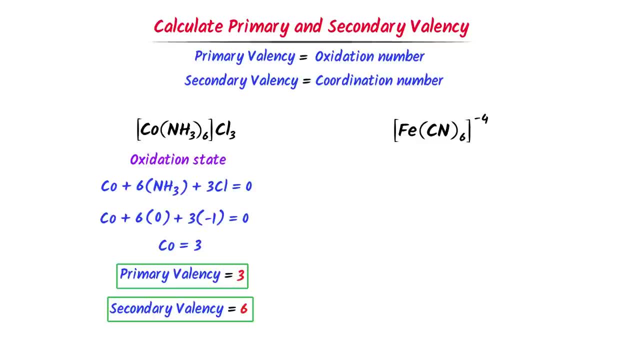 Secondly, in case of this molecule, I find the oxidation state of iron- I write iron plus 6 and 2- Cn- equals negative 4, because the overall charge on this coordination compound is negative 4.. We know that the oxidation state of Cn is negative 1. I write iron plus 6 and 2- negative. 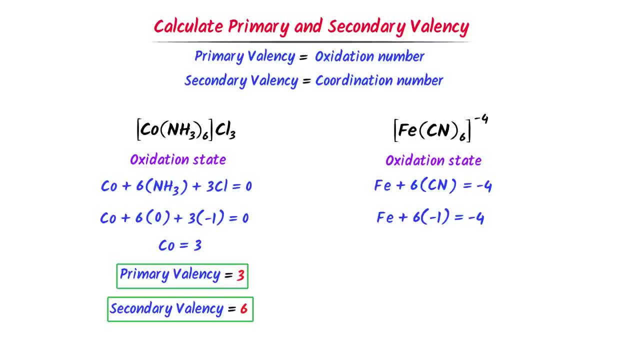 1 equals negative, 4. After calculation I get positive. 2. The oxidation state of iron is positive: 2. So the primary valency of iron is positive. 2. Here there are 6 ligands of Cn. The coordination number is 6. So the secondary valency of iron is 6.. Therefore, using this, 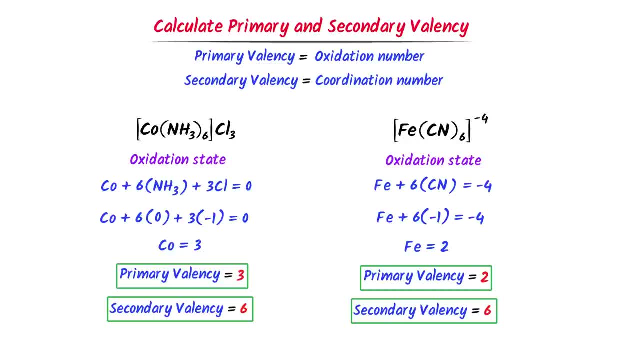 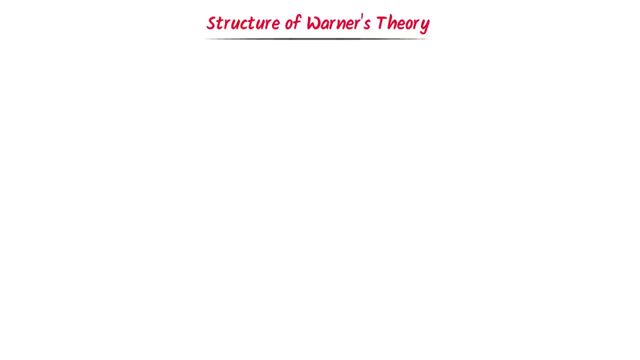 trick. we can easily calculate the primary and secondary valencies of a central metal atom. Now let me teach you the structure of Warner's theory. Well, consider these four coordination compounds. I write cobalt and I draw 6 lines as the octahedral structure. 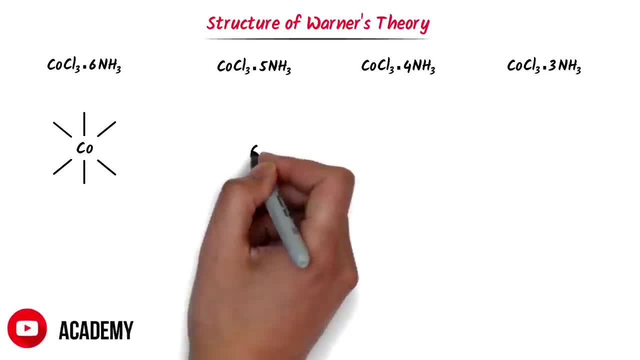 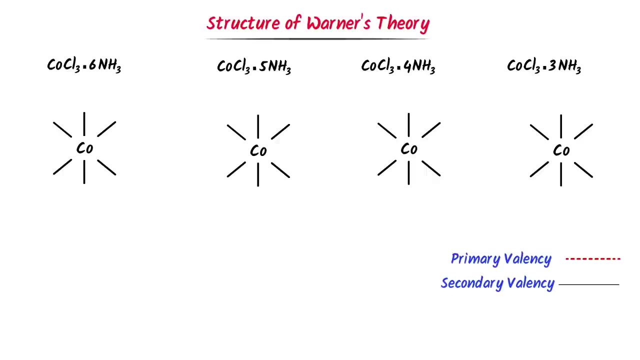 Similarly, in case of these 3 compounds, I write cobalt and I draw 6 lines as the octahedral structure. We know that primary valency is denoted by dots and secondary valency is denoted by line. Now listen carefully. these are 6 molecules of NH3. 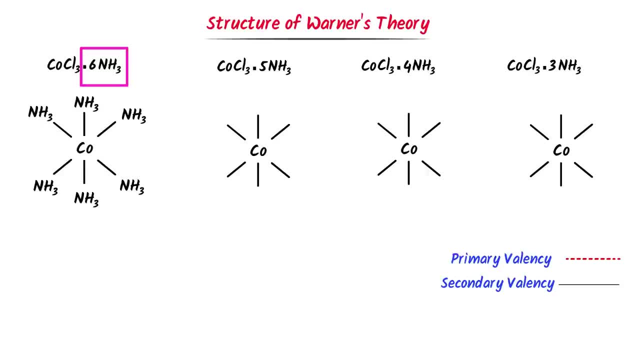 I draw these 6 molecules of NH3 around the central atom cobalt. Now I take these 3 ions of chlorine. they satisfy the primary valency. so I randomly draw 3 dot lines And I put 3 chlorine ions around cobalt. 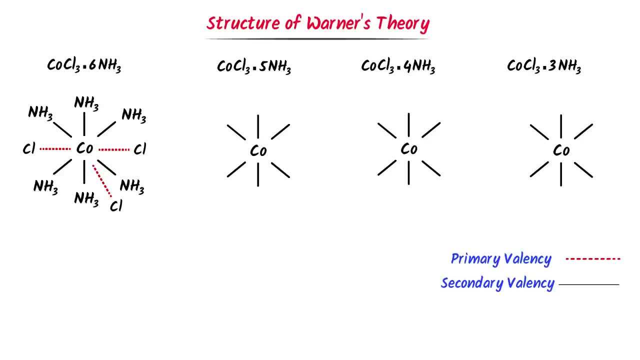 Remember that you can draw this dotted line in any direction around the central atom. Secondly, in this coordination compound there are 5 cobalt ions around the central atom. Similarly, in case of these 5 molecules of NH3, I write them around the central atom. 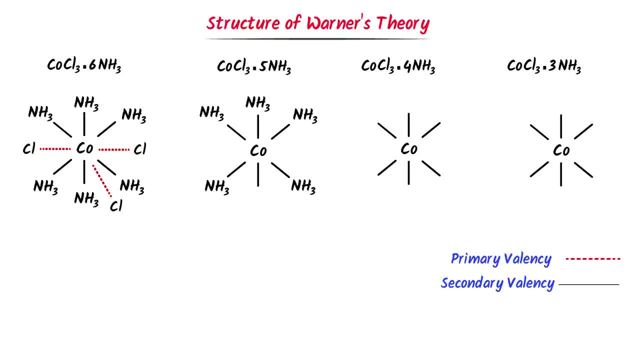 Now one secondary valency is left behind, so I place 1 chlorine here. Remember that this chlorine can fulfill the secondary valency and primary valency of the central metal atom. I draw 2 dotted lines and I place 2 chlorine. Similarly, I write 4 NH3 around the central atom. 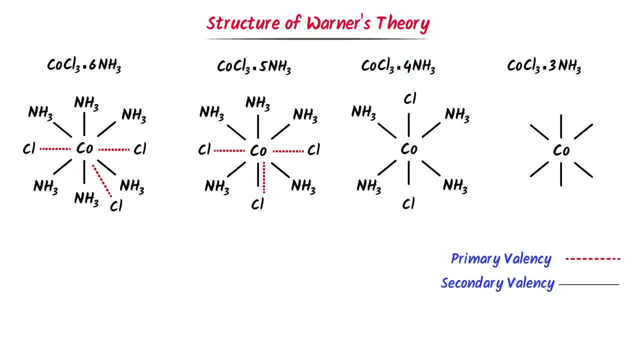 I write here 1 chlorine and 1 chlorine. Here these 2 chlorine act as a primary valency and secondary valency. I draw 1 dotted line and I write chlorine. Lastly, I write 3 NH3 around the central atom. 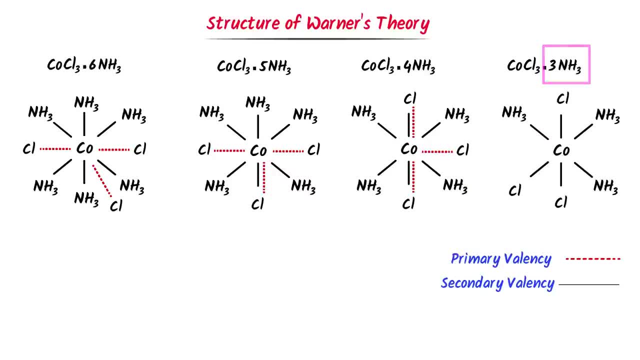 I write chlorine, chlorine and chlorine Here. these 3 chlorine act as a primary valency and secondary valency. Now Warner-Baba added silver nitrate to each of these coordination compounds. After chemical reaction he got different amount of products. 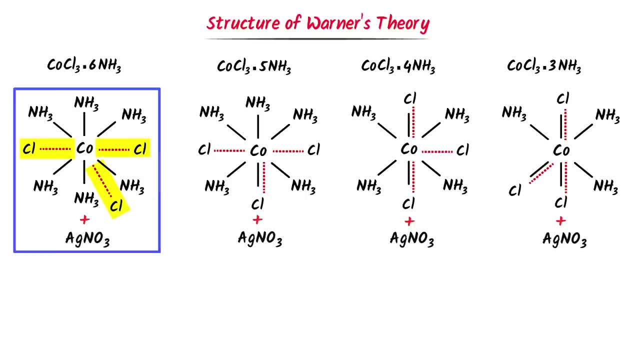 In case of this molecule, these 3 dotted lines mean 3 chlorine are out of coordination sphere. Let me repeat it: These 3 dotted lines mean 3 chlorine are out of coordination sphere. Thus, here, 3 moles of silver chloride is formed. 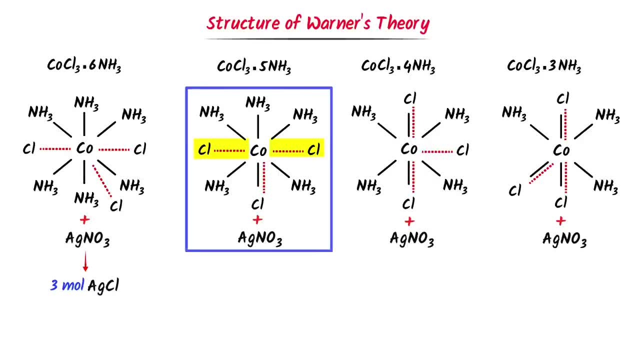 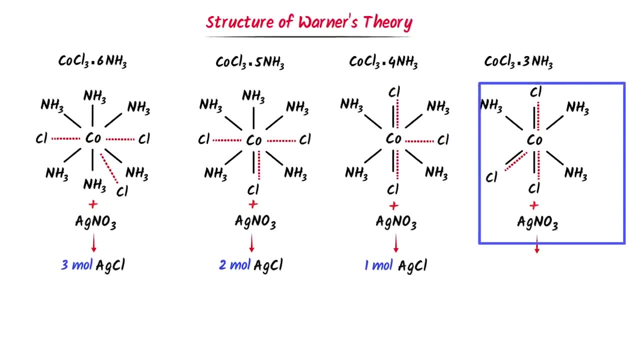 In this case, 2 chlorine are out of coordination sphere, So 2 moles of silver chloride are formed. In this case, only 1 chlorine is out of coordination sphere, So 1 mole of silver chloride is formed. In case of this coordination compound, no chlorine is out of coordination sphere. 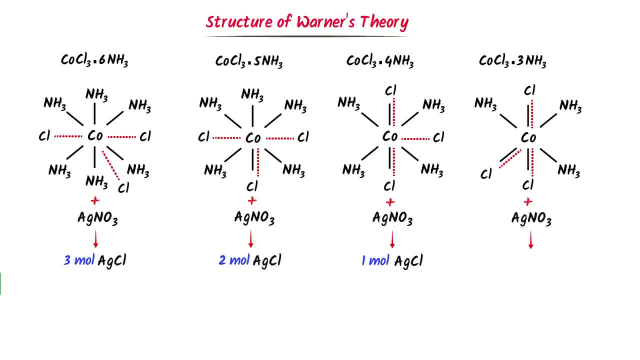 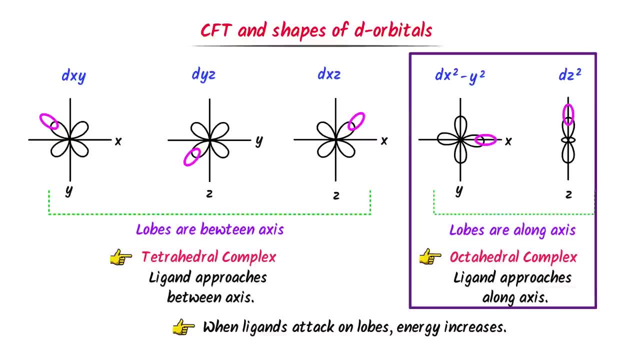 Cobalt- NH3, 6 square bracket, Cl 3.. The structure of this compound is Cobalt: NH3, 6 square bracket Cl 3.. The structure of this compound is Cobalt- NH3, 6 square bracket Cl 3.. along x-axis, energy of only d- x squared minus y squared and d z squared increases. We know that. 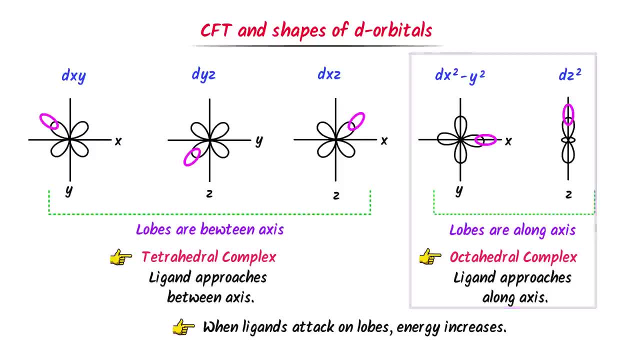 it only happens in octahedral complex. Secondly, if we gain a tax between x-axis, energy of d x y, d y z and d x z increases. We know that it only happens in tetrahedral complex. To summarize this whole concept, we say that in case of octahedral complex, the energy of these 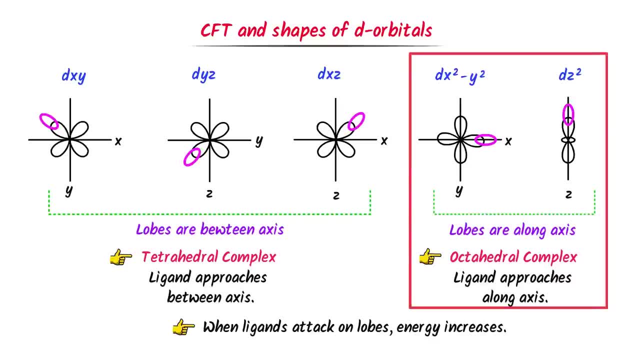 two orbitals increases and the energy of these three orbitals decreases, While in case of tetrahedral, the situation is opposite: The energy of these three orbitals increases and the energy of these two orbitals decreases. Let's note down all these important points. 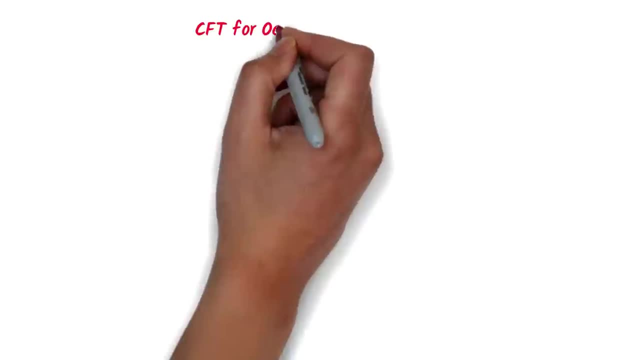 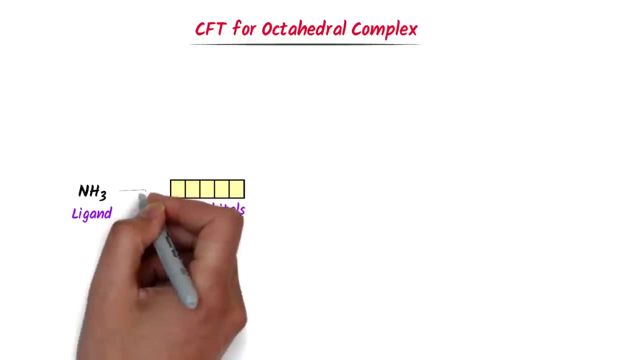 Now let me show you how to calculate the energy of these three orbitals. Let me teach you the trick to draw the structures of CFT for octahedral. Well, consider these five degenerate d orbitals. The average energy of these five orbitals increases when ligand. 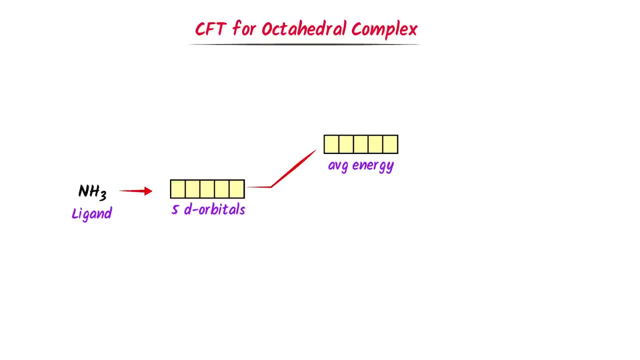 approaches near the d orbitals. A lot of students are confused that why energy of d orbital increases. I teach them a very simple example. I always say when you are in danger, you are addressing the energy of d orbitals. You are addressing the energy of d orbitals, You are. 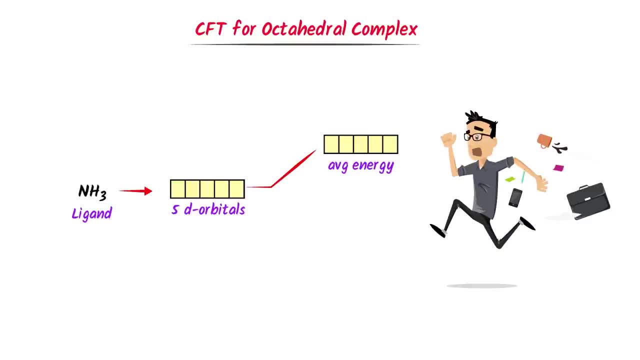 addressing the energy of d orbitals. When you are in danger, you are addressing the energy of d orbitals. Similarly, when ligand approaches toward these orbitals, they get excited and their average energy increases. Remember that I used the term average energy After interaction: the five d: 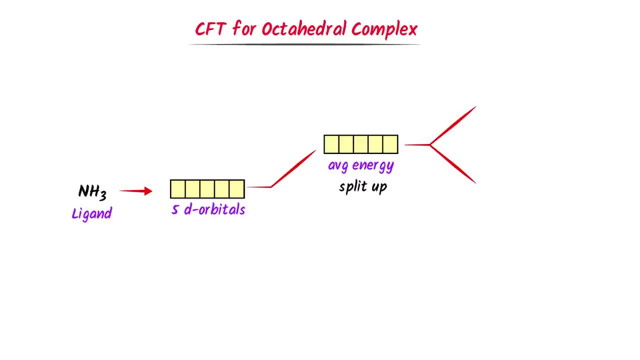 orbitals split into two sets. We have already learned that in case of octahedral complex, the ligand approaches along axes. The energy of d x square minus y square and d z square increases, While that of d x y, d y z and d z, d x z decreases. 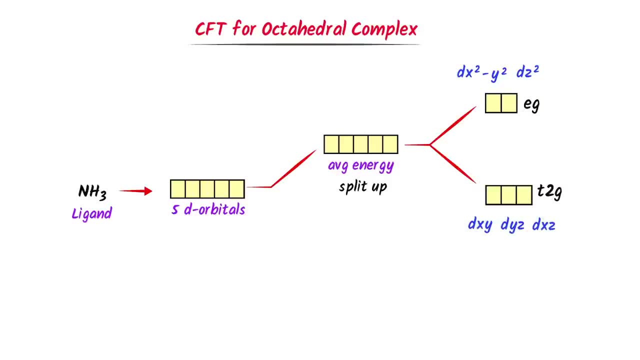 And we call these three orbitals as d2g. This is the energy gap between them, which we call CFS, crystal field splitting. Here we can see that the energy of these two orbital increases from the average energy level. So I write positive 0.6 delta. Secondly, the energy of these three orbital. 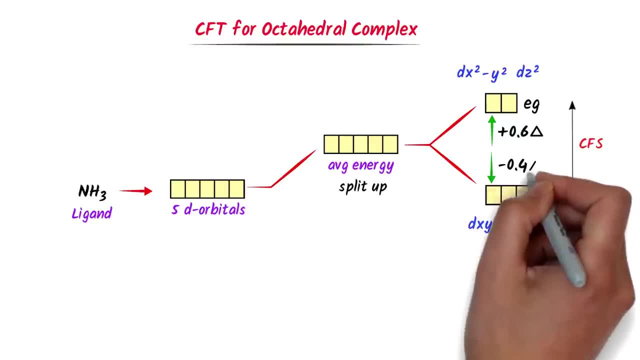 decreases. So I write negative 0.4 delta. So the value of eg equals positive 0.60 and that of t2g equals negative 0.40.. Thus noted down this diagram of octahedral, Now let me teach you. 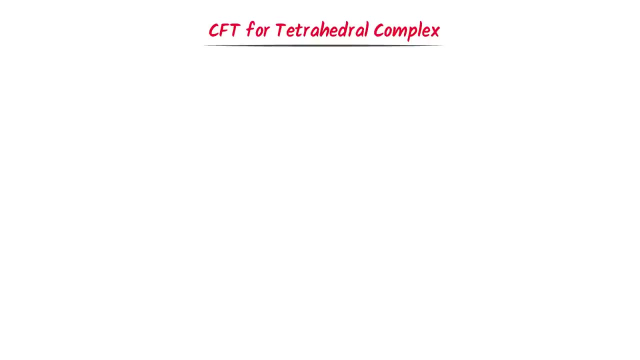 crystal field splitting. So let me teach you crystal field splitting. So let me teach you the crystal field theory for tetrahedral. Well, consider these five degenerate d orbitals. The average energy of these orbitals increases when a ligand approaches nearer them After. 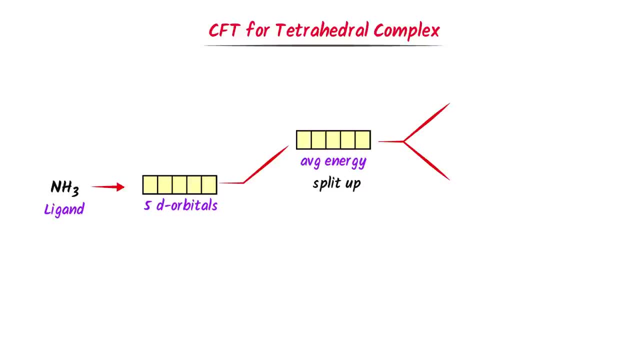 interaction the five d orbitals splits into two sets. We have already learned that in case of tetrahedral, complex ligand approaches between axes. So the energy of d, x, y, d, y, dxz increases and that of dx square minus y square and dz square decreases. Remember that. 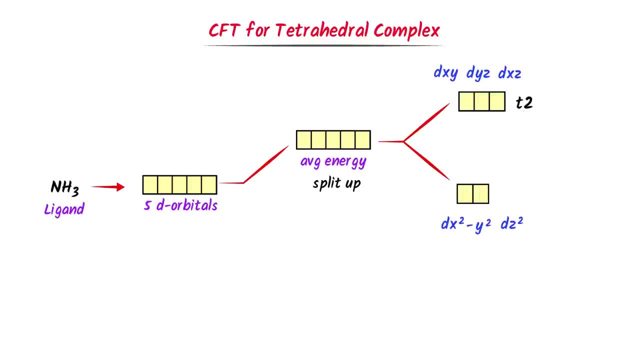 in case of tetrahedral, this is t2 set and this is e set of orbitals. We do not try g with them. Secondly, this is the energy gap, or CFS, between these two sets of orbitals. Thirdly, the energy. 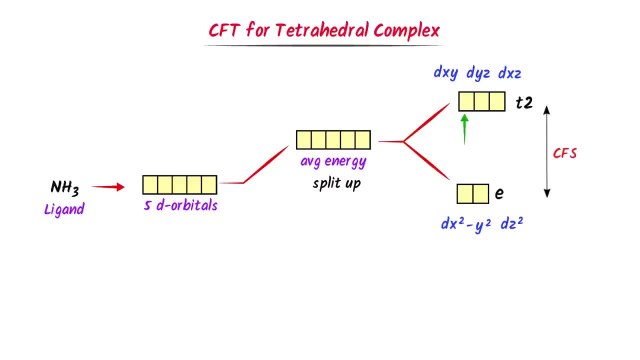 of these three orbital increases from average level. it is positive 0.4 delta and the energy of these two orbital decreases from average level, so its value is negative 0.60 delta. Thus the value of t2 equals positive 0.40 delta and that of e equals negative 0.60 delta. 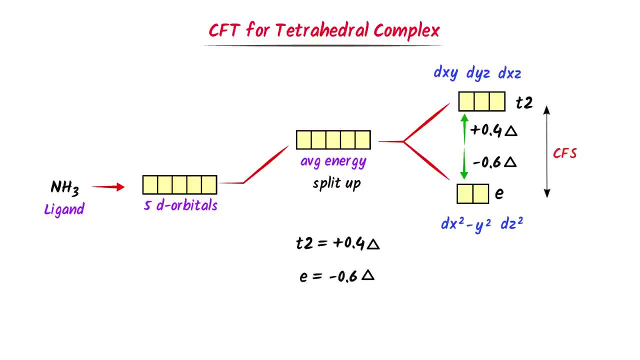 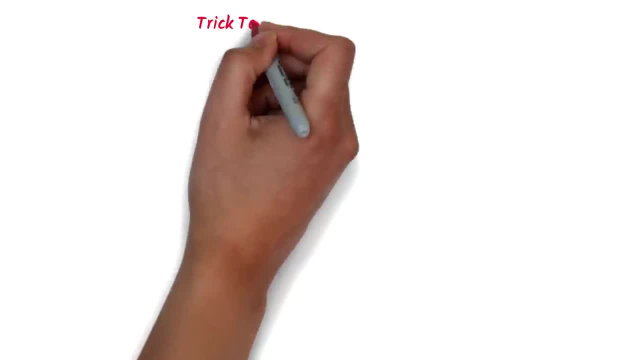 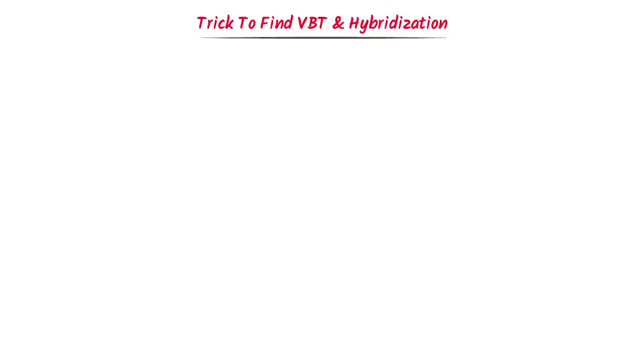 Therefore, using this trick, we can easily write CFT for octahedral and tetrahedral complex. Finally, let me teach you my personal trick of VBT and hybridization of coordination compounds, which I have already explained in my previous video. Now consider this coordination compound. 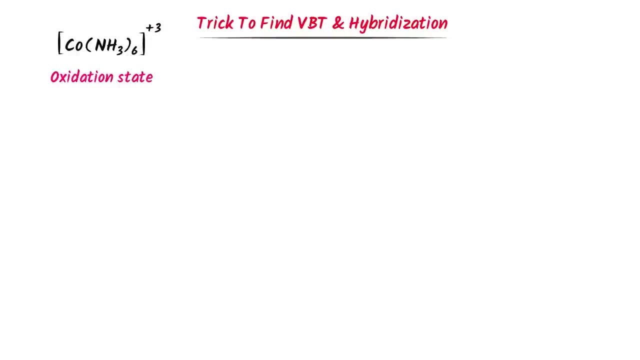 Firstly, I find the oxidation state of a central atom. I write: cobalt plus 6- NH3 equals positive. 3. Our cobalt plus 6- NH3 equals positive. 3. Accumulation of a boolean formed by insulating space occurs. 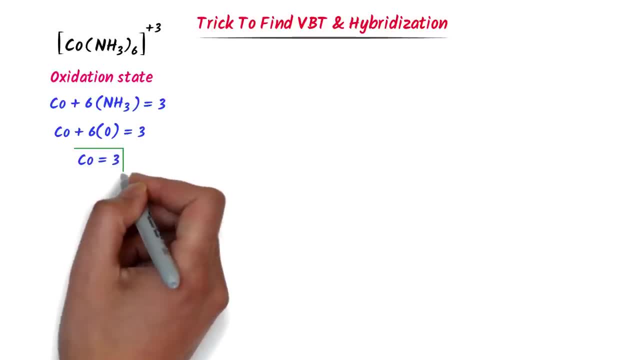 I vector포: equalsflows andugeos, musicbirdx- equals positive, 3. I get cobalt: equals positive, 3. So the oxidation state of cobalt is positive, 3. It replaced by a Boolean chemistry. Secondly, I find the number of electrons of cobalt. 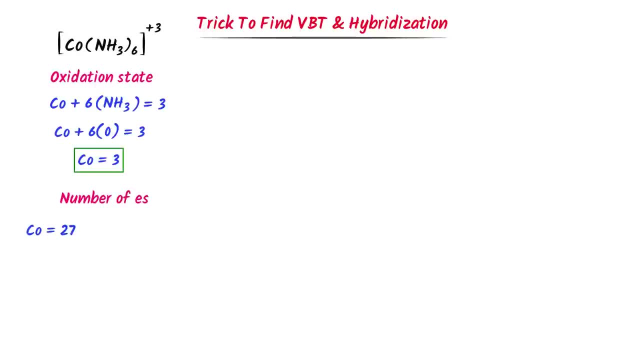 We know that the atomic number of cobalt is 27.. Now listen carefully. I always subtract oxidation state of central atom minus 1 from the atomic number of central atom. Let me repeat it: I always subtract oxidation of central atom minus 1 from atomic number of central atom. 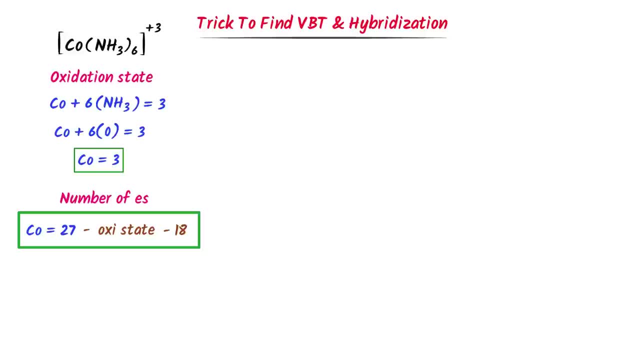 This means that my cobalt comes from the atomic number of swear atom plus 3.. subtract oxidation state of a central atom minus 18 from the atomic number of central atom. here the oxidation state of cobalt is positive, 3, so I write cobalt. 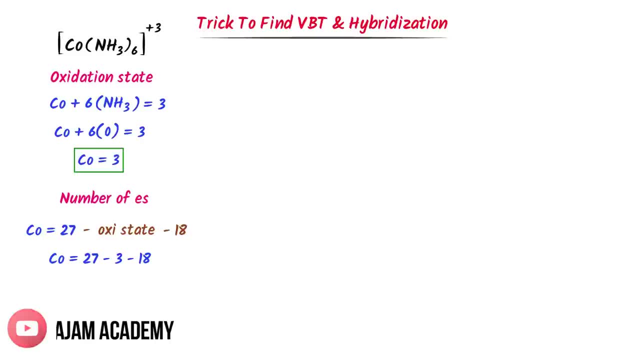 equals 27 minus 3 minus 18, I get 6 electrons. now we can see that here the ligand is NH 3 and it is a strong ligand. remember that in case of a strong ligand, the electrons of the central atom get paired, while in case of weak. 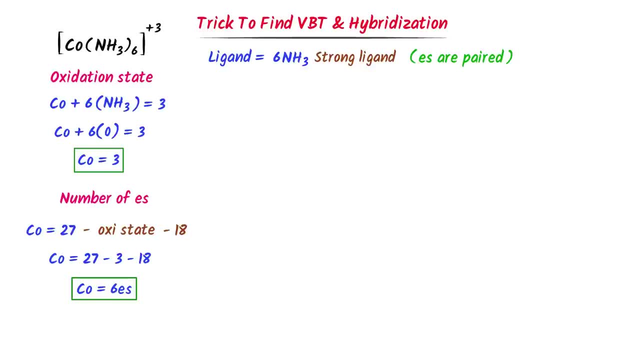 ligand. the electrons of the central atom do not get paired. now I use the police trick. I say: DSP, doctor, we know that D has five orbitals, S has one orbital, D has three orbitals and D has five orbitals. now listen carefully. I take the. 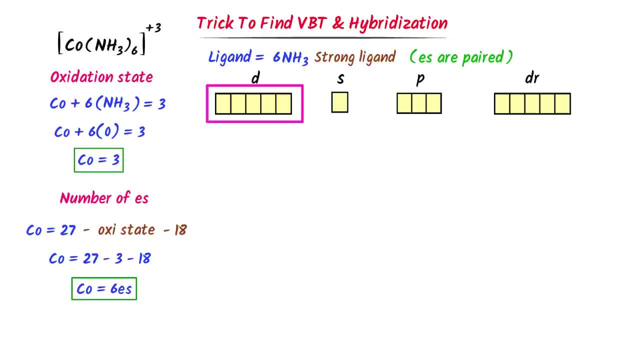 six electrons of central atom and I place it in this D orbital: 1, 2, 3, 4, 5, 6. I have paired these electrons because the ligand is strong. we can see that there are six ligands of NH 3, so I select six.